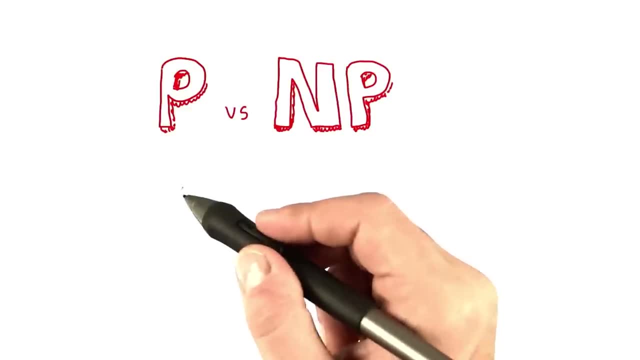 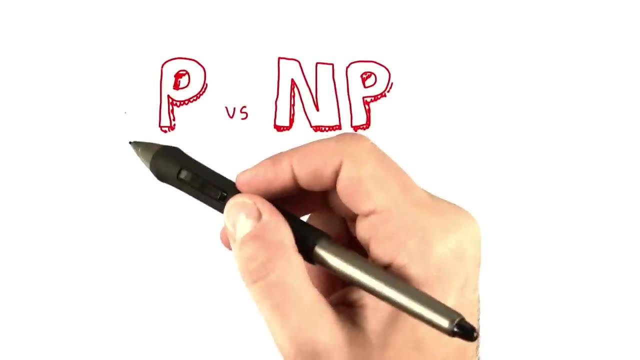 which would mean that a normal deterministic RAM without the if better function is just as powerful as one that has this function, which of course seems a bit strange because our intuition of course tells us that having this if better function is superimposed on the if better function. So if you have a non-deterministic RAM without the if 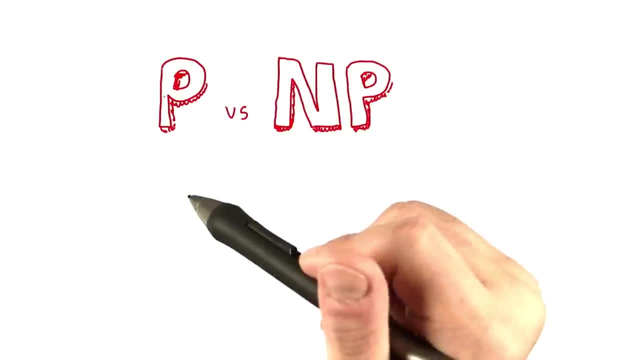 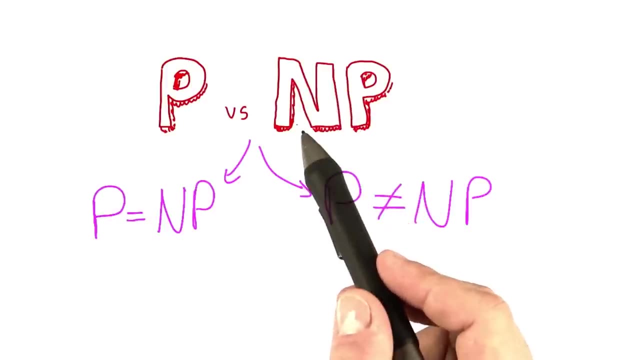 better function. this is super, super powerful and should somehow make a difference. So the cool thing is there's only two possibilities: Either all NP complete problems can be solved in polynomial time, which would essentially mean that P equals NP, So any problem that can be solved. 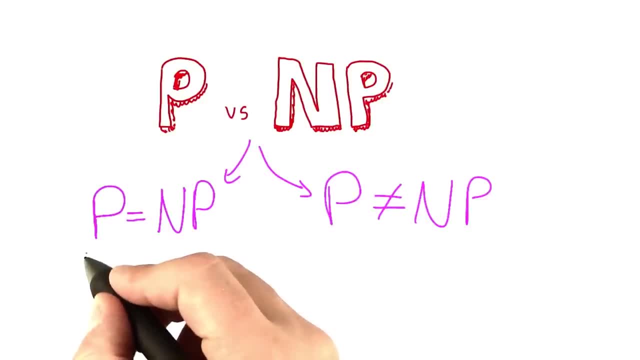 in polynomial time on a non-deterministic RAM can be solved in polynomial time on a deterministic RAM, Or in other words, a deterministic RAM is just as powerful as a non-deterministic one, Or that could be the other case. That is no NP. complete problem can be solved in polynomial time. So P does not equal NP. There are 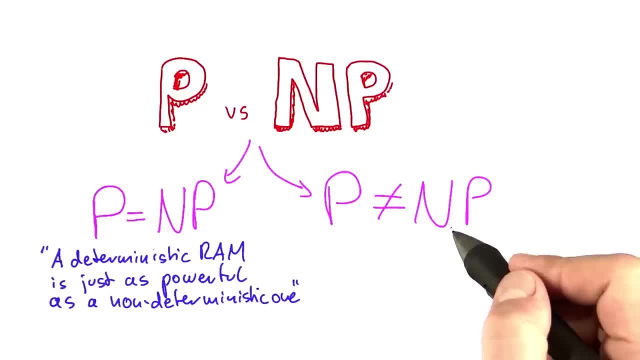 certain problems that you can solve in polynomial time if you have the if better function available. but you cannot solve them in polynomial time if you don't have this function. So basically you'd say P does not equal NP is the same as saying that the if better function is really powerful. 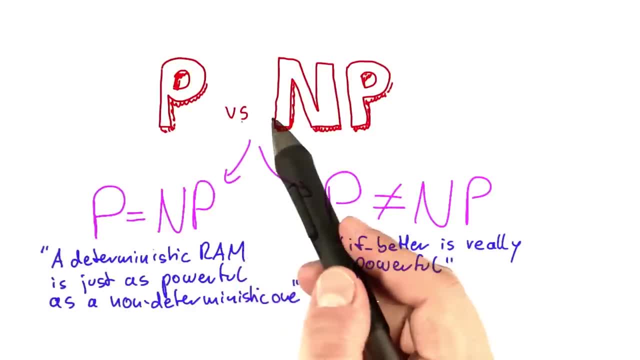 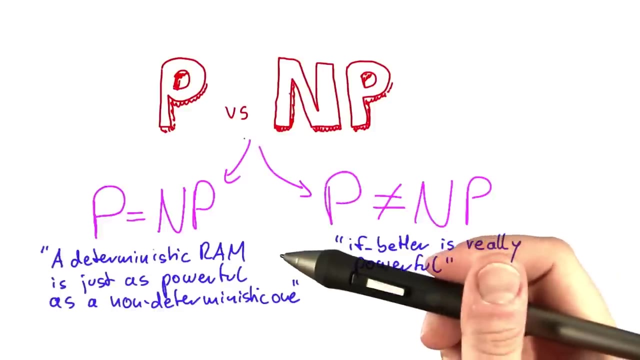 So which one is it? And that question is the famous P versus NP, Because the thing is we don't know, Nobody knows. Asking this question here, if P equals NP or P does not equal NP is a problem that is decades old and yet nobody has been able to figure it. 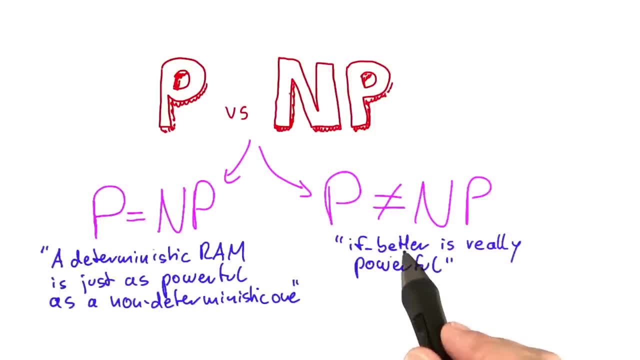 out Now, given how powerful this, if better, function is. remember when I introduced it to you. it seemed like this magic function that could solve all of our problems. Many computer scientists nowadays believe that P does not equal NP, But nobody has been able to prove it. On the other hand, also nobody has been able to find a 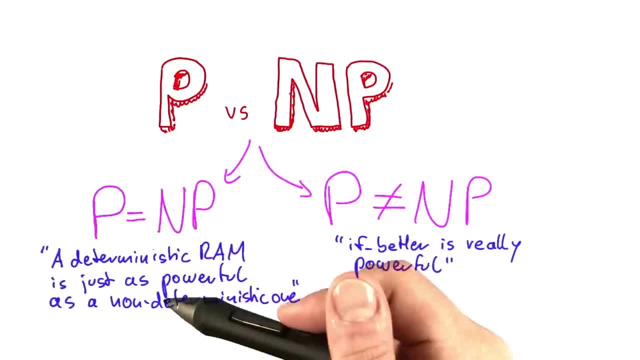 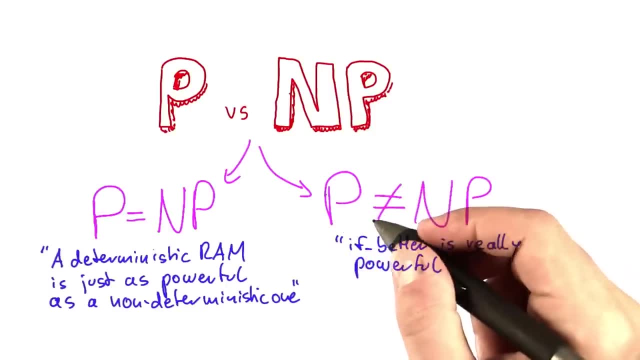 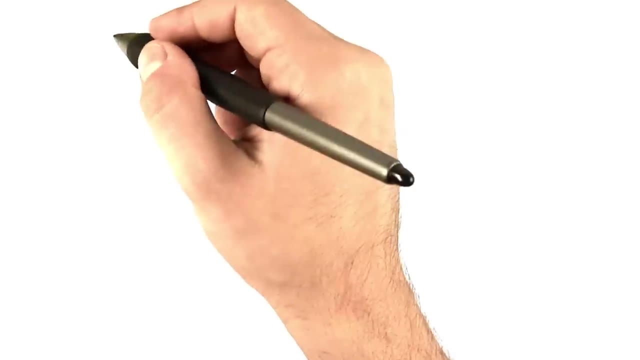 polynomial time algorithm for any single NP complete problem, despite literally thousands of practically relevant NP complete problems being out there. Now let's think a little bit of how you could resolve this question. So how could you show that P equals NP or P does not equal NP? And we'll